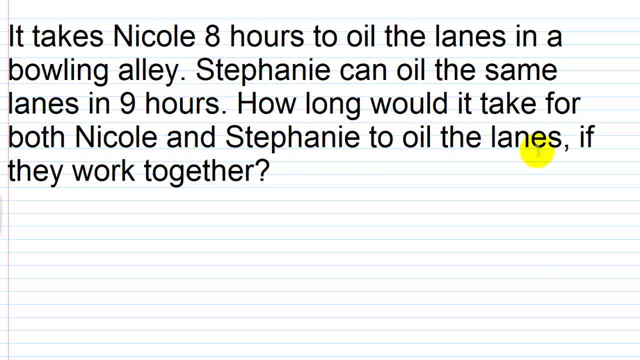 How long would it take for both Nicole and Stephanie to all the lanes if they work together? So I think for most problems like these, they're. they're very, very simple. Okay, they're very, very simple. Let's start by just going back and just highlighting some stuff. It takes Nicole eight. 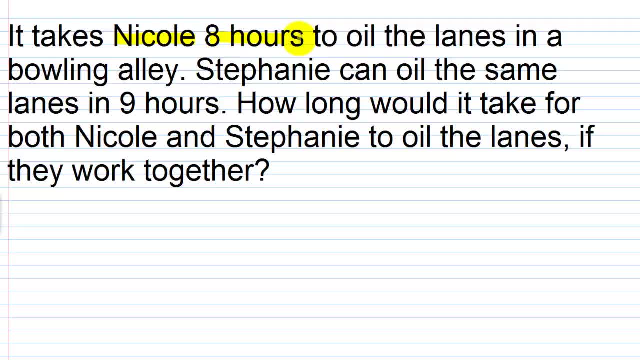 hours to all the lanes in a bowling alley. Then Stephanie can all the same lanes, so the same lanes in nine hours. and then our question here, which I want to highlight, is how long would it take for both Nicole and Stephanie to all the lanes if they work together? So we want to assign a 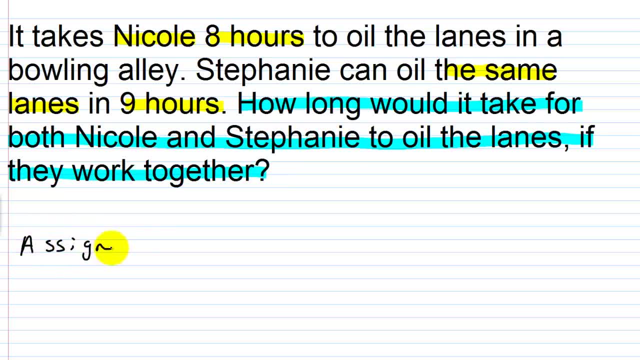 variable. here Let's let- and we always use x. So let's just try, let's. let's say let's let Z equal the number of hours for Stephanie and Nicole to complete the job, Alright, and so let's call that a prologue. Let's throw in a function. 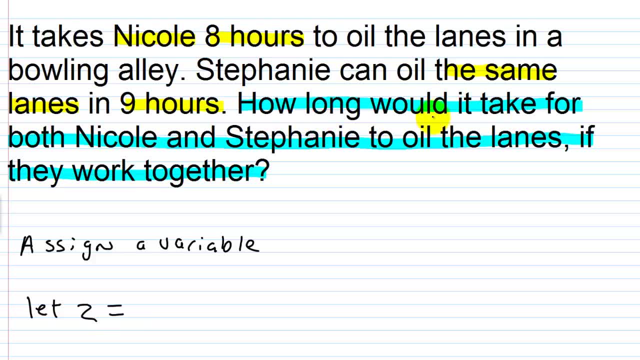 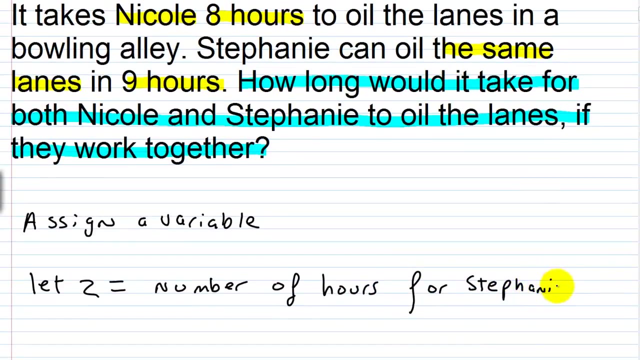 the job together, because that's what we're trying to figure out right, how long would it take for both Nicole and Stephanie to all the lanes if they work together? so Z will be equal to the number of hours for Stephanie and Nicole to complete the job together. so once we have our variables on, we want to set up 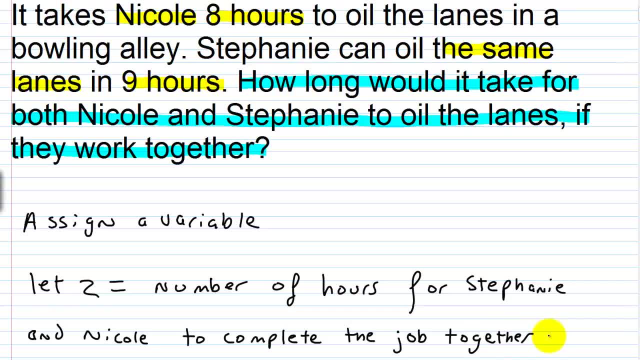 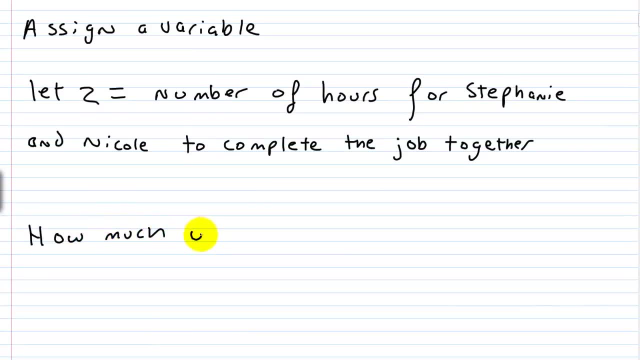 an equation, and it's really really very, very simple to set up an equation here. if the first thing you need to understand is think about the unit of time, here it's in hours. so if I think about how, how, how much work, and this is what you always need, to ask yourself how much work is. 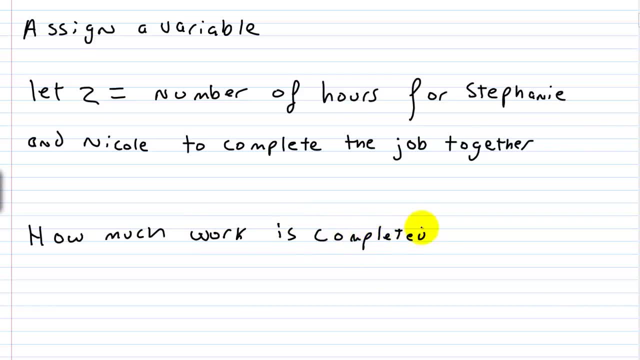 completed by each person, would say per one unit of time. so in this case we're dealing with hours, right, because the time is given to us in hours, right? if you go through the problem again, Nicole takes 8 hours to all the lanes and Steffany takes 9 hours to all the lanes. so if we 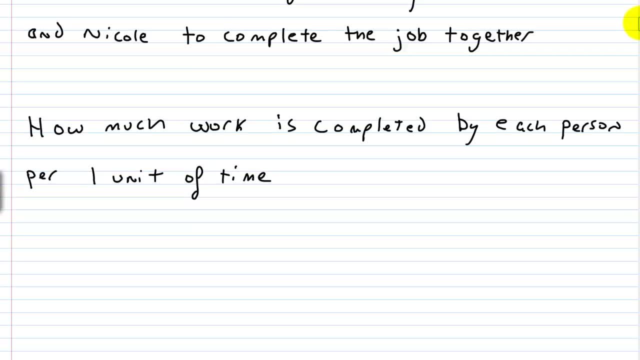 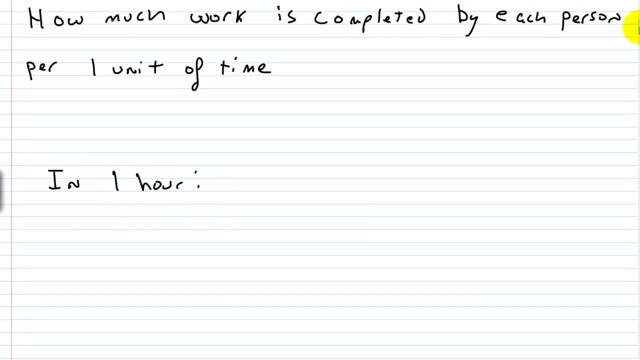 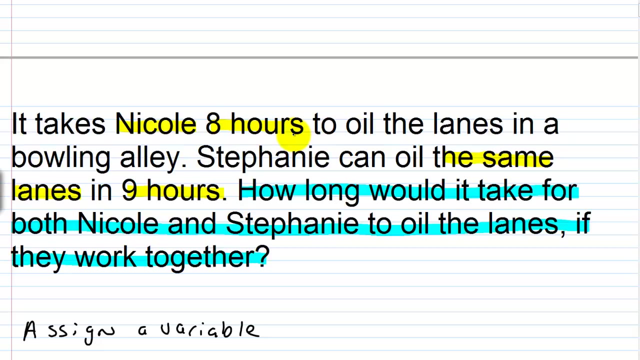 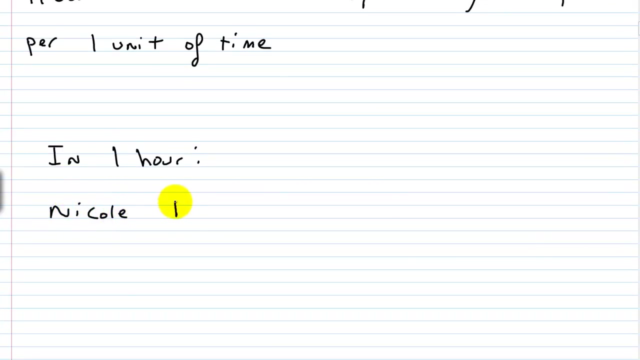 so if we think about one unit of time, we would ask ourselves the question: in one hour we want to say what happens. so when in one hour Nicole takes eight hours to, in one hour she's completed 1 eighth of that job. so in one hour Nicole has completed 20 hoursOK. 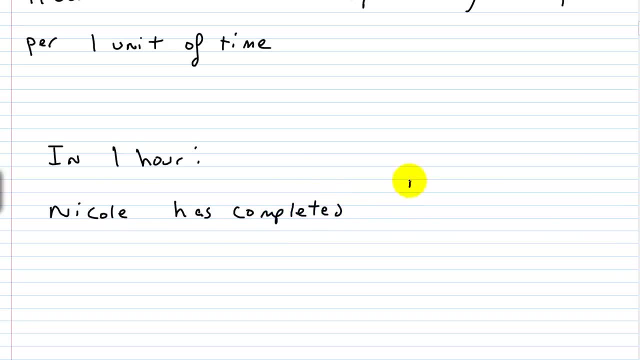 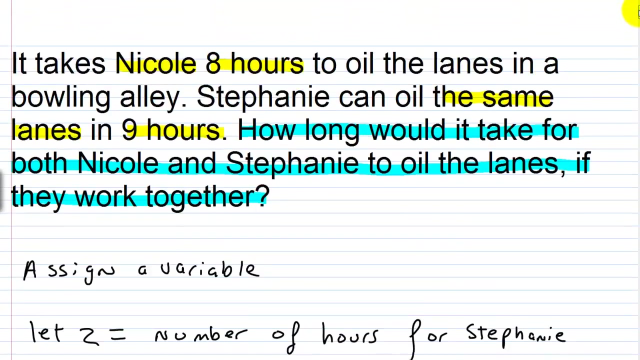 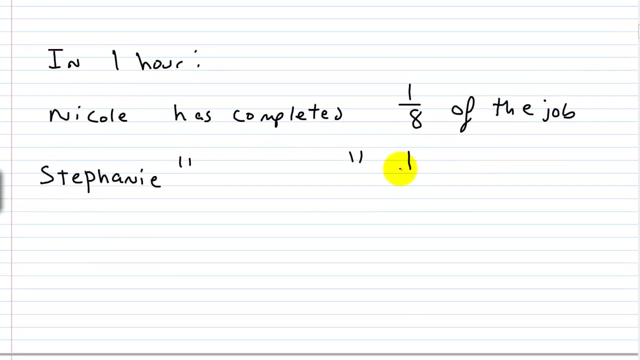 Tolerance. one-eighth of the job. and stephanie has completed. what if we go back up here? takes her nine hours, so in one hour she's done one night, right. one-ninth of the job. so what does this tell us? if they work together over the course of an hour? 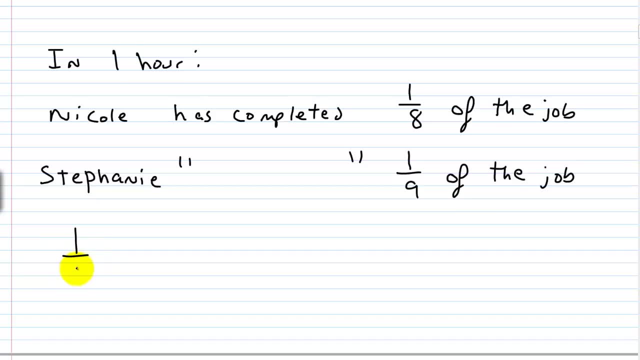 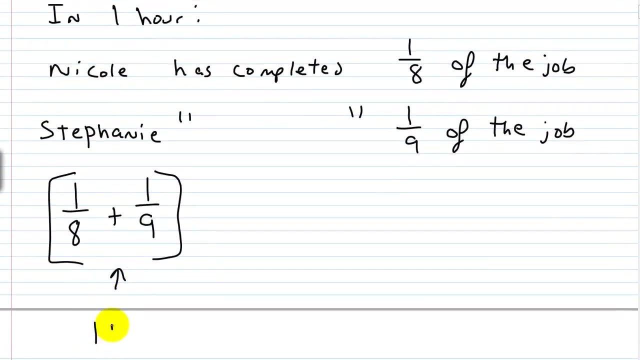 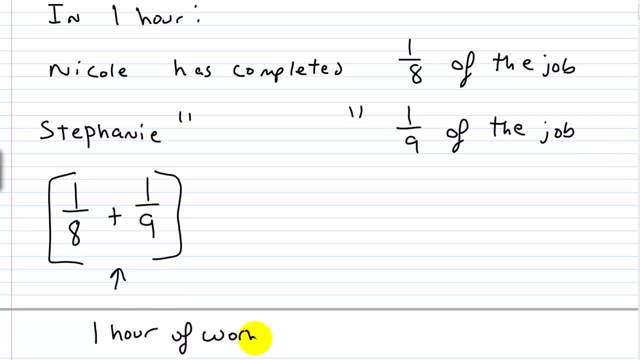 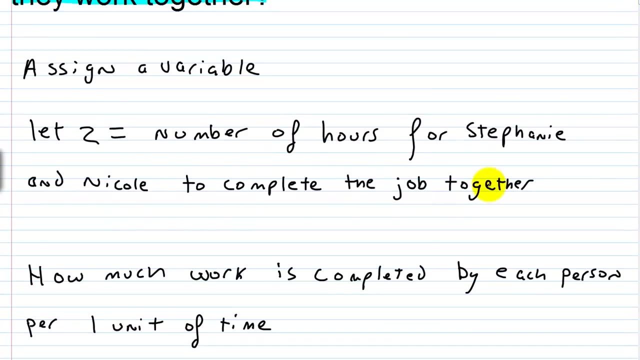 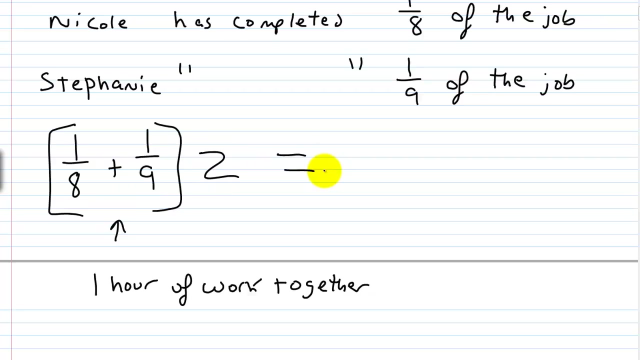 hour of work together. so then, if I multiply this by the number of hours that they work right to complete the job, which we said was Z, right, Z is the number of hours for Stephanie Nicole to complete the job together. so we're multiply this by Z, this should be equal to what it's gonna be equal to one right. 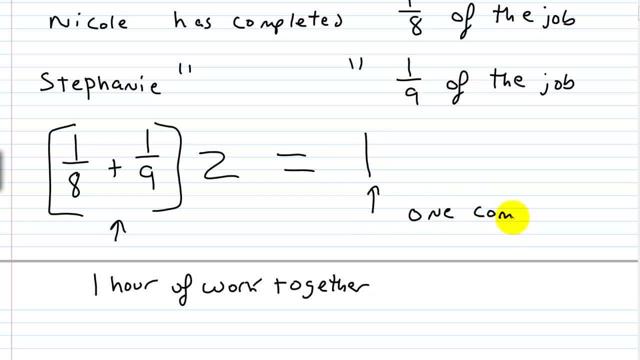 and this one represents one completed job. okay, so now we have our equation. we have one hour of work together. right, that represents Nicole and Stephanie working together. that's what they've accomplished, times Z, which is the number of hours they work together. so you multiply those two together and you're. 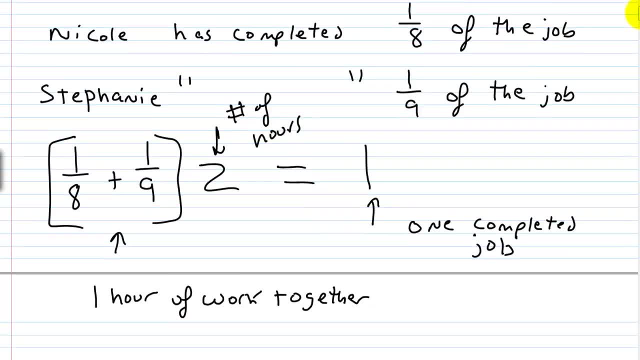 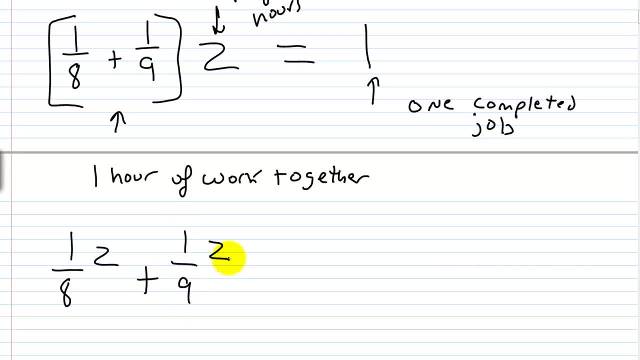 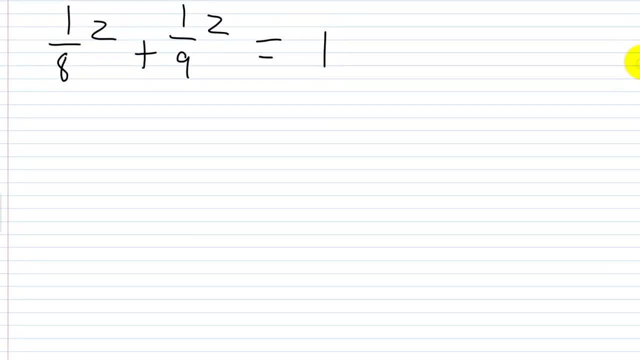 gonna get one completed job. so let's solve this equation and find out what Z is. so we'll have 1, 8 times Z plus 1, 9 times Z, and all I did was use. the distributive property is equal to 1, so we'll find the LCD here. 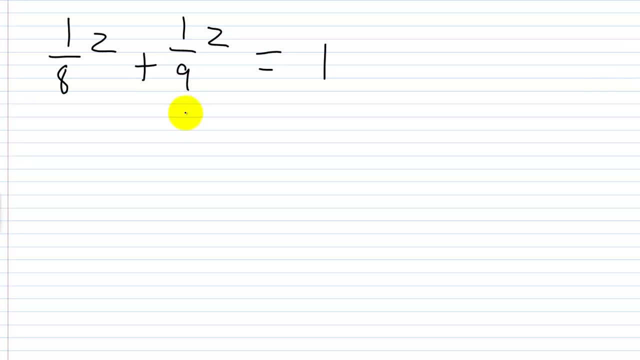 right, we're just working with some fractions and the LCD. if you think about this, 9 is 3 times 3, 8 is what? 2 to the 3rd power. so it should be 8 times 9 or 72, so I'll have 72 times 1, 8 Z plus. 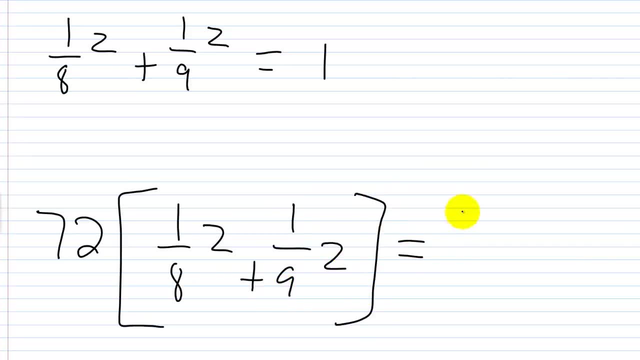 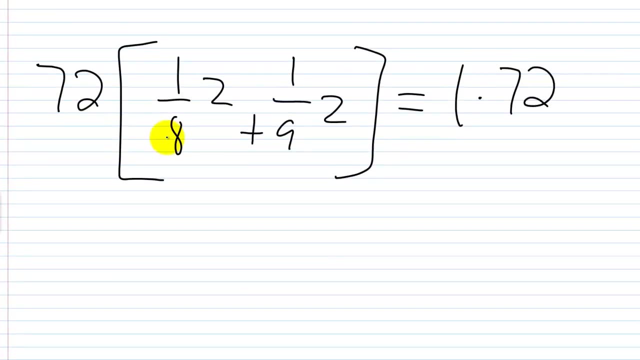 1, 9 Z equals 1 times 72, and I continue that down here- 72 times 1, 8 Z. 72 divided by 8 is 9, so you'll have 9 Z then plus- I'll write this up here- 72 times 1, 9 Z. 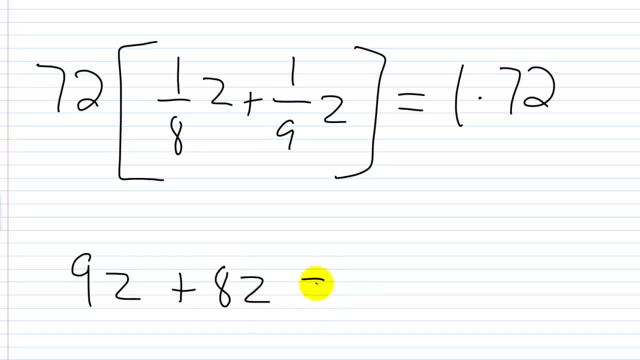 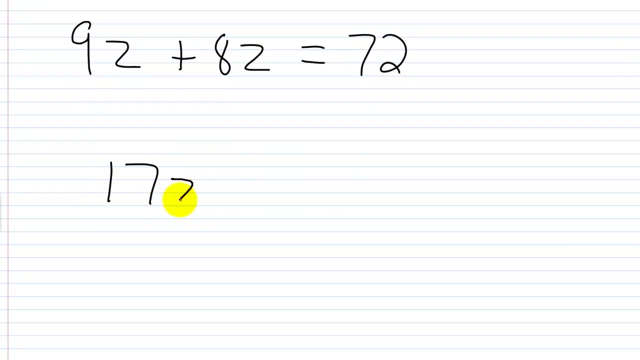 72 divided by 9 is 8. so you'll have 8. Z equals 1 times 72, which is 72, and so you get 9 Z plus 8 Z, which is 17. Z equals 72. divide both sides of the equation by 17. that's gone. you'll have a 1 there. you'll have a z equals. 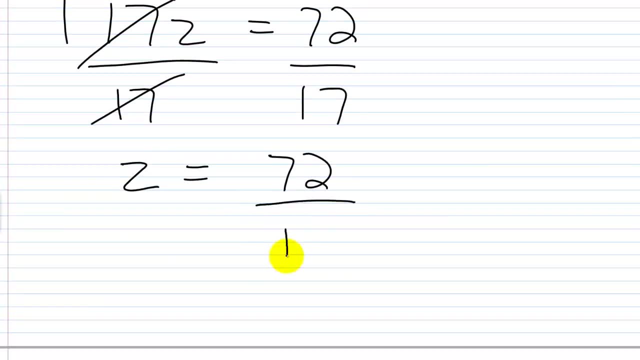 72 over 17.. So this is the answer, and I know it's not a, you know, nice pretty answer, but it takes 72 over 17 hours for them to work together and complete that job, which is oiling the lanes. and in decimal form you punch up 72 divided by 17 on a calculator, you'll get approximately 4.24. 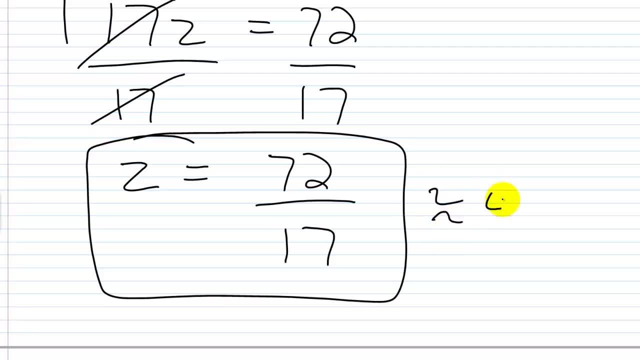 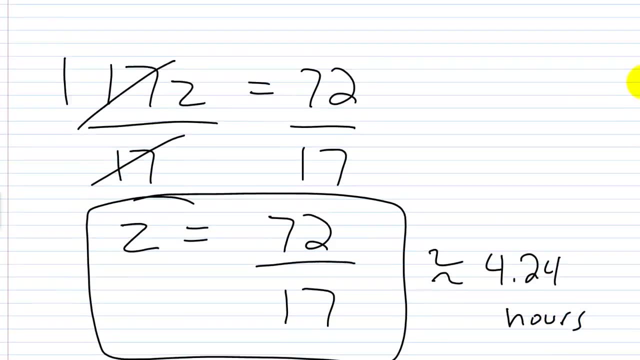 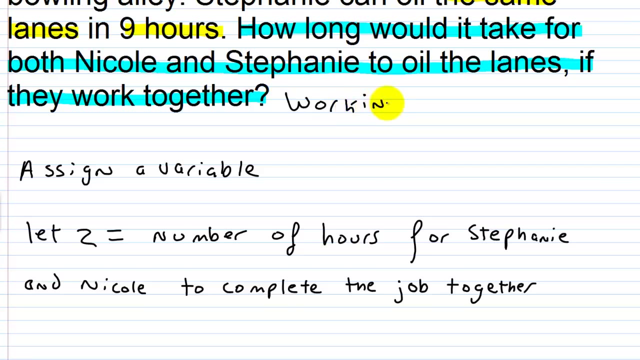 okay. so we'll say this is approximately 4.24 hours. So now that we have our answer, let's write a nice little sentence. nice little sentence. so we'll say that working together it takes about because, remember, our answer in decimal form is an approximation. 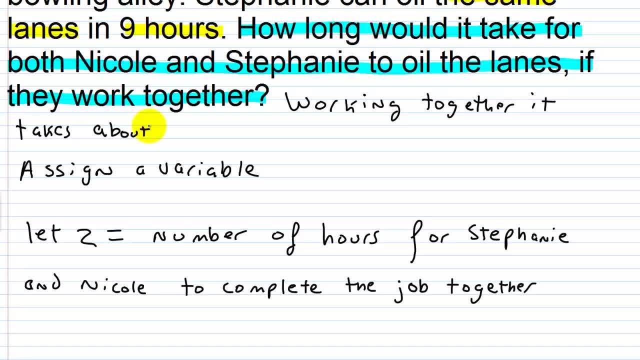 it's an approximation, so I'm going to put 4.24 hours to complete the job. Okay, so, working together it takes about 4.24 hours to complete the job, So we're going to put 4.24 hours to complete the job. 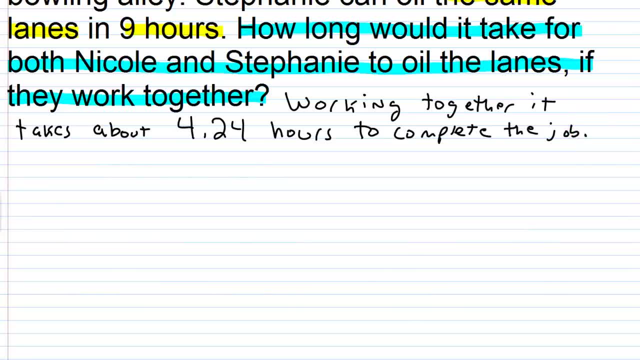 So let's check to make sure that we're accurate, And all we really have to do is check our equation that we set up, Because, again, we know that in an hour, Nicole's done 1, 1⁄8 of a job.